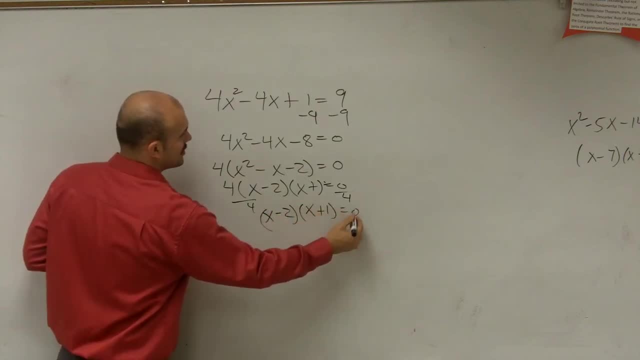 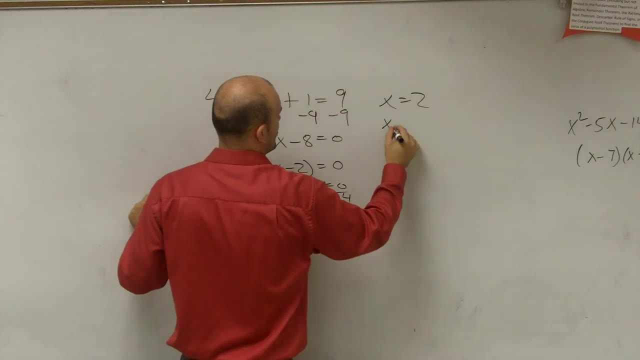 could say: x minus 2 times x plus 1 equals zero. Therefore x minus 2 equals zero, x plus 1 equals zero. So we could say: x equals 2 and x equals negative 1.. Now, I did that really. 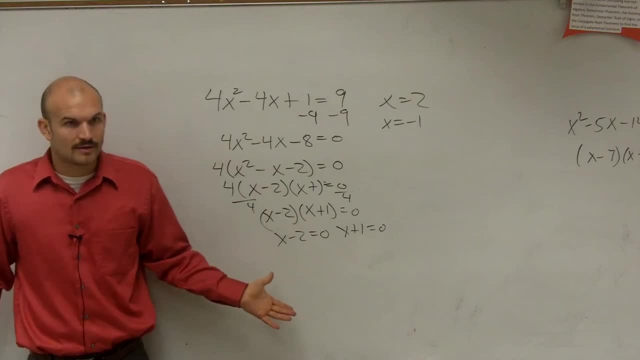 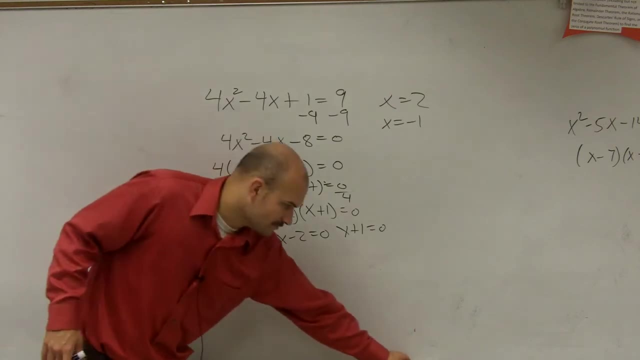 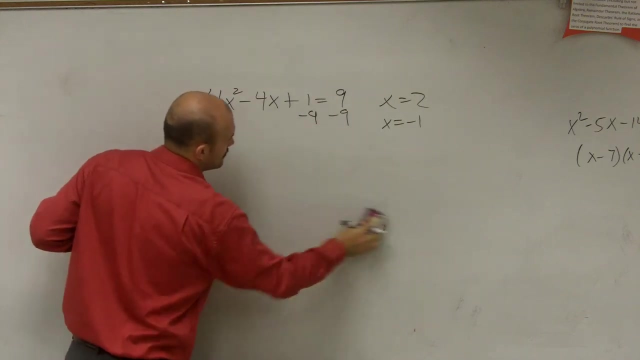 quickly, because we've already gone through how to do all that right, And not always is that going to be factorable. So what happens if it's not factorable? So let's pretend that when you subtract 8, that you don't have a factorable equation. The next thing you guys want to look at. 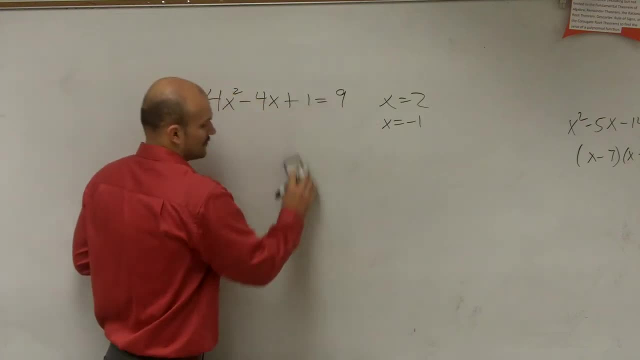 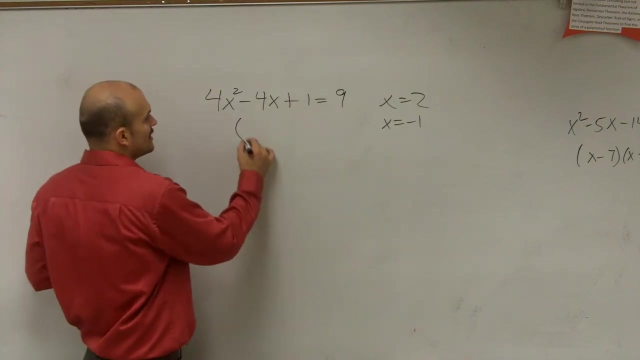 is to determine: is this a perfect square triangle? Is this a perfect square triangle? Is this a perfect square trinomial? Because if it's a perfect square trinomial, I don't have to set it equal to zero Meaning. can I write this as a factor? squared, All right. So what that really? 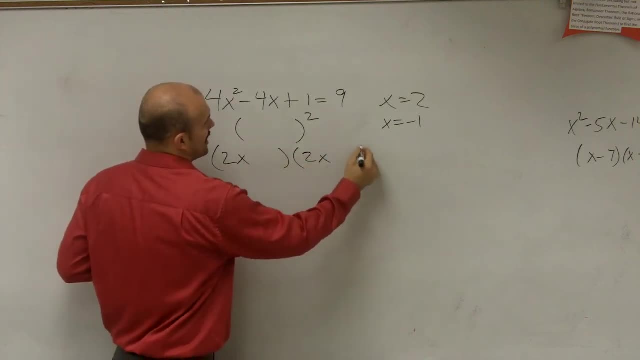 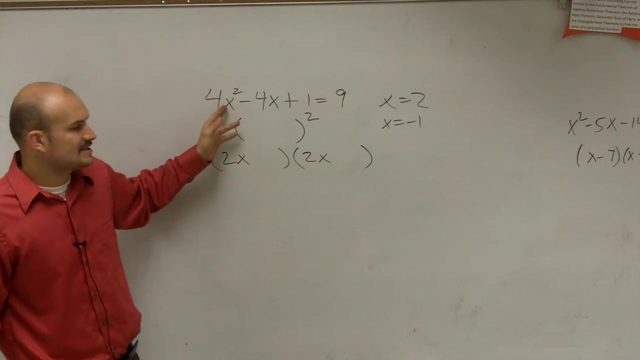 means is the same factor multiplied by itself. So obviously we have to use 2x and 2x, because you can't use 4x and x. So I have 2x times 2x is going to give me 4x squared. Then I have to have: 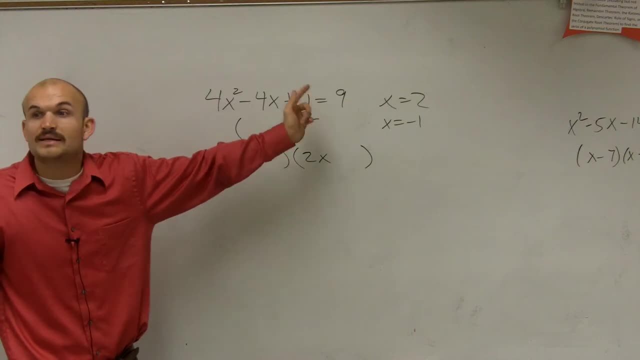 what two numbers multiply to give you 1?. It could be 1 and 1, or it could be negative 1 and negative 1.. However, I know that I'm going to use negative 1 and negative 1 because my middle term is. 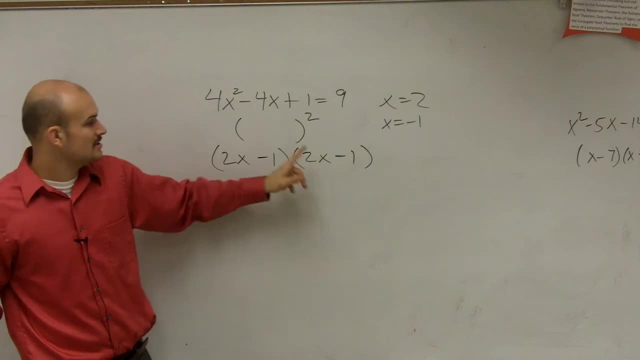 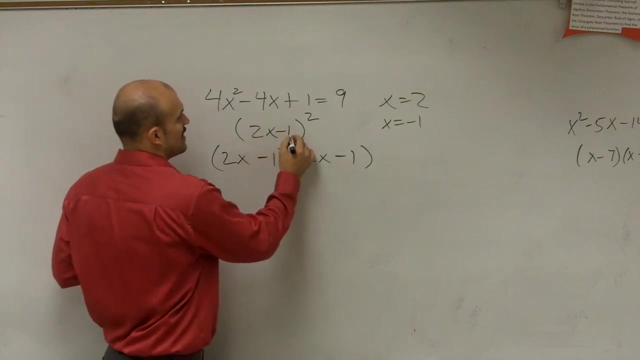 negative Because negative 1 times 2x is negative 2x and 2x times negative 1 is again 2x. Add those up together, you're getting negative 4x. So my answer is negative. 2x minus 1 squared equals 9.. 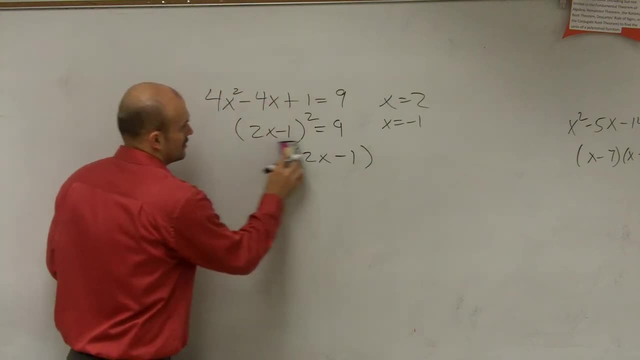 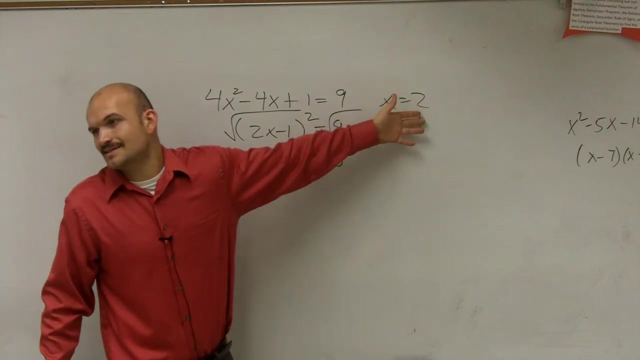 Can we solve that without using the zero product property? Yes, of course we can. How do we solve that? Inverse operations. So therefore, you have 2x minus 1 equals plus or minus 3.. So then, once you have plus or minus 3, we already know. I kind of did the 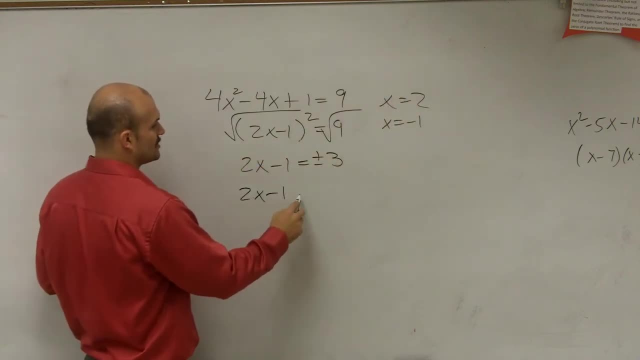 problem twice. but we already know what you'll do is. I'll just set it up differently. I'll do: 2x minus 1 equals negative 3, and 2x minus 1 equals positive 3.. So therefore, you just add 1.. 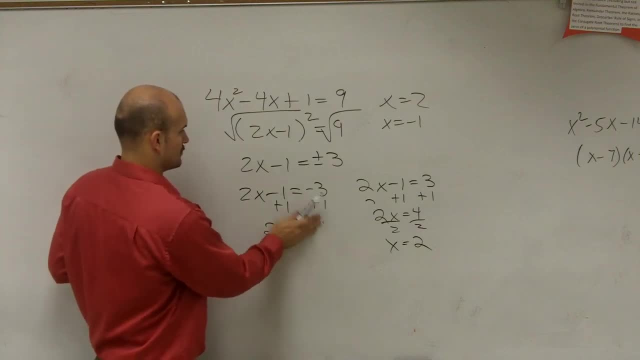 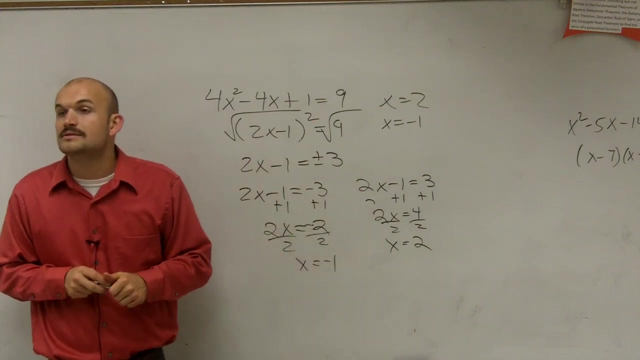 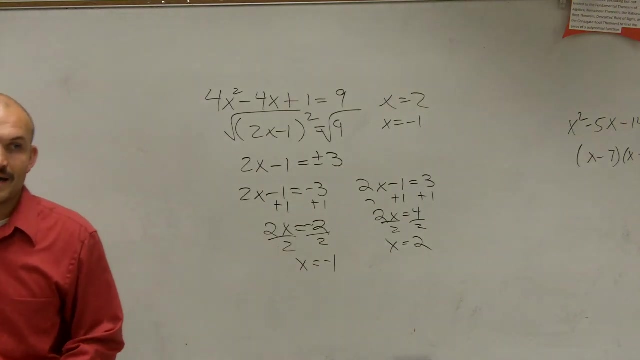 And there you go. Oops, I tried to do both in there, Negative 2.. So by doing it by the square root method, you guys notice I get the exact same answers: Yes, question. So always, guys, you can always look to that first factoring form. but a lot of these problems are not going to be factorable. 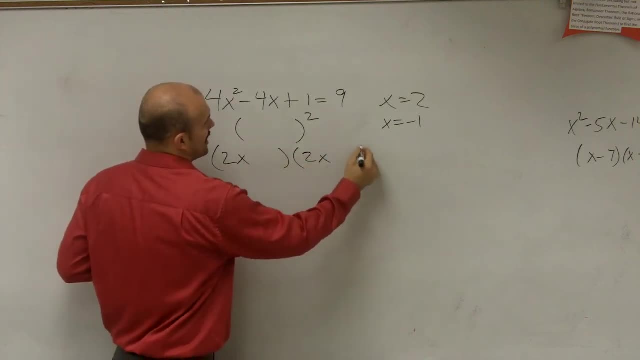 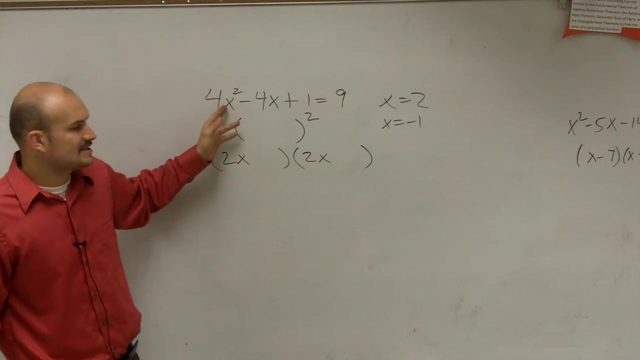 means is the same factor multiplied by itself. So obviously we have to use 2x and 2x, because you can't use 4x and x. So I have 2x times 2x is going to give me 4x squared. Then I have to have: 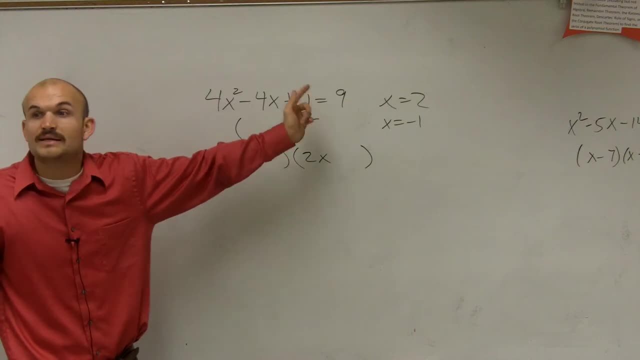 what two numbers multiply to give you 1?. It could be 1 and 1, or it could be negative 1 and negative 1.. However, I know that I'm going to use negative 1 and negative 1 because my middle term is. 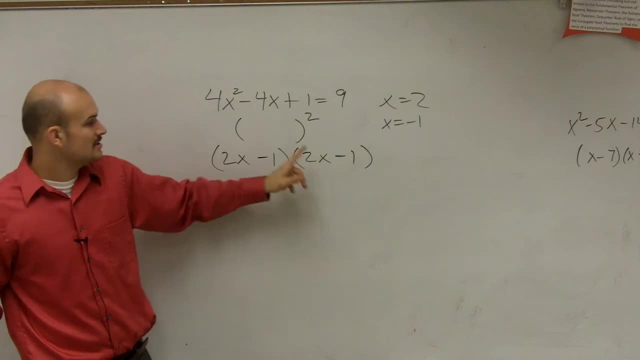 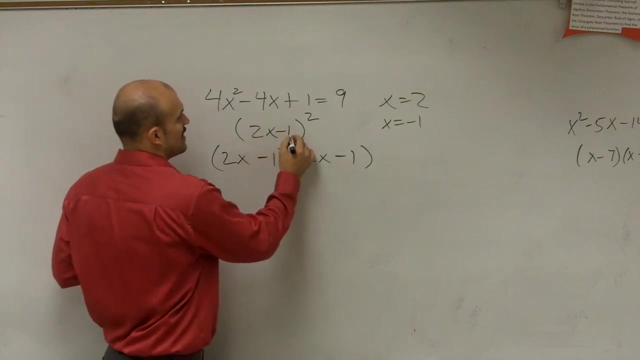 negative Because negative 1 times 2x is negative 2x and 2x times negative 1 is again 2x. Add those up together, you're getting negative 4x. So my answer is negative. 2x minus 1 squared equals 9.. 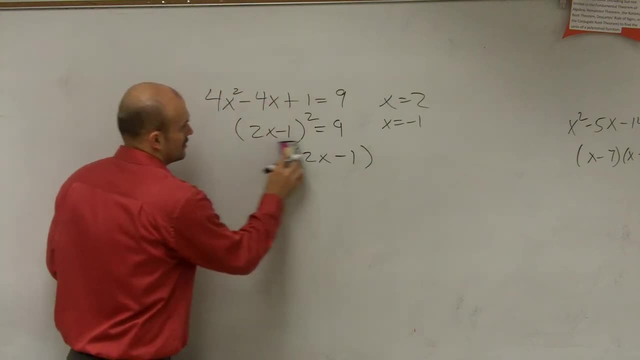 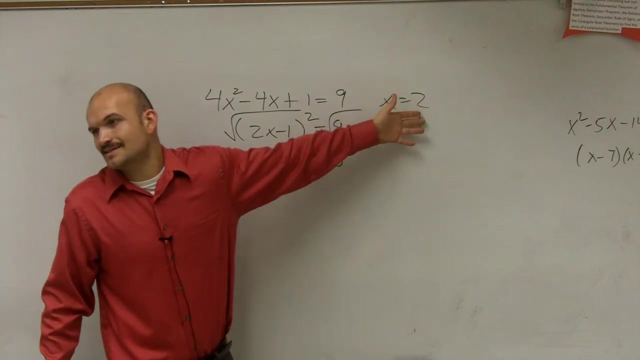 Can we solve that without using the zero product property? Yes, of course we can. How do we solve that? Inverse operations. So therefore, you have 2x minus 1 equals plus or minus 3.. So then, once you have plus or minus 3, we already know. I kind of did the 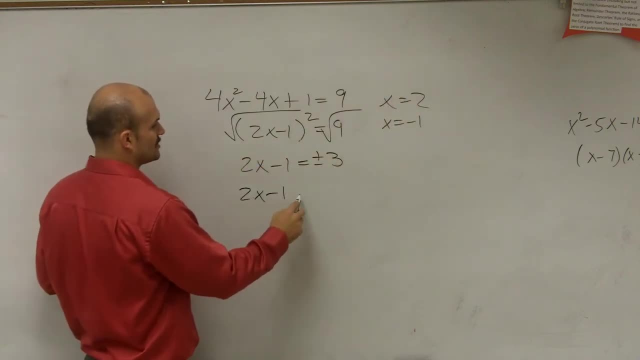 problem twice. but we already know what you'll do is. I'll just set it up differently. I'll do: 2x minus 1 equals negative 3, and 2x minus 1 equals positive 3.. So therefore, you just add 1.. 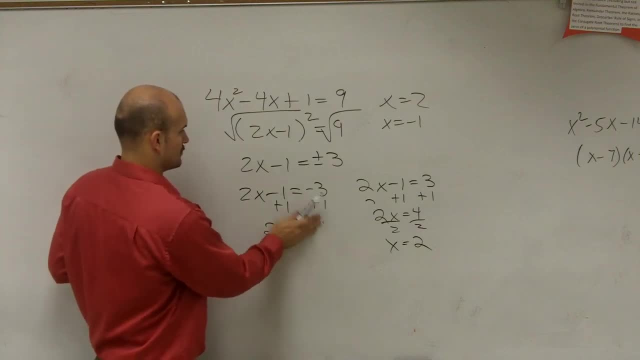 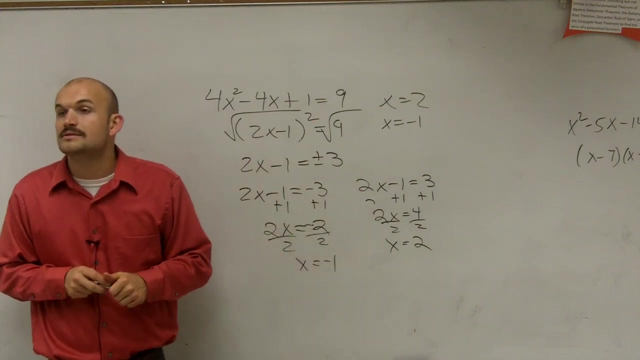 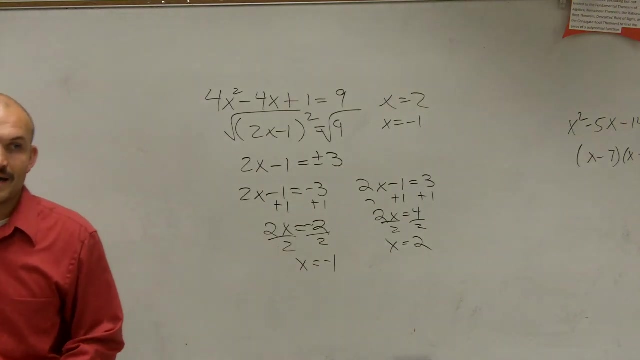 And there you go. Oops, I tried to do both in there, Negative 2.. So by doing it by the square root method, you guys notice I get the exact same answers: Yes, question. So always, guys, you can always look to that first factoring form. but a lot of these problems are not going to be factorable. 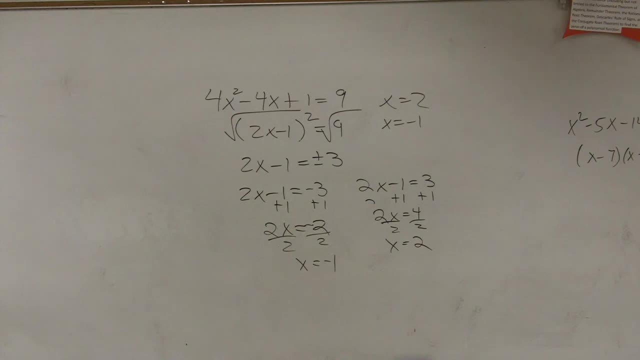 as is, so you might have to go back and use the square root method. Thank you.